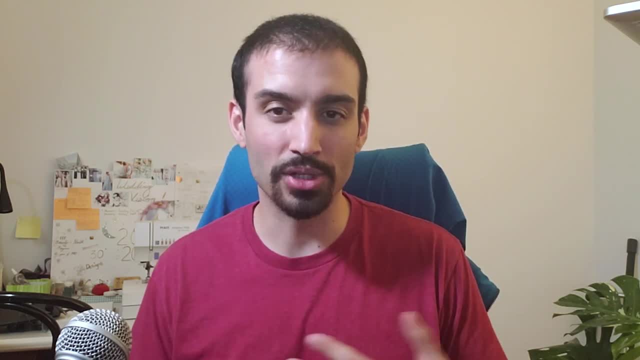 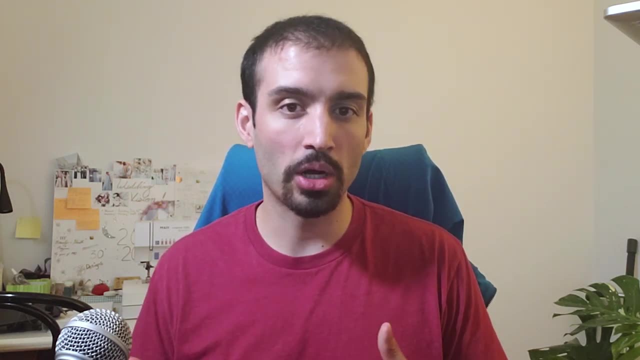 refactoring is important is because software is meant to change, It's meant to evolve and last for long periods of time, And this is especially relevant if you're working for large organizations where you have, like a couple core services that are ingrained in how the system works And over. 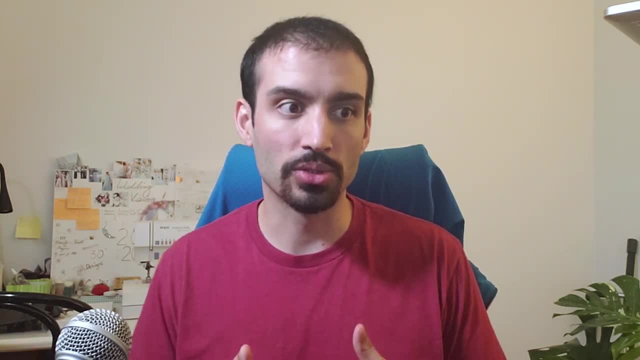 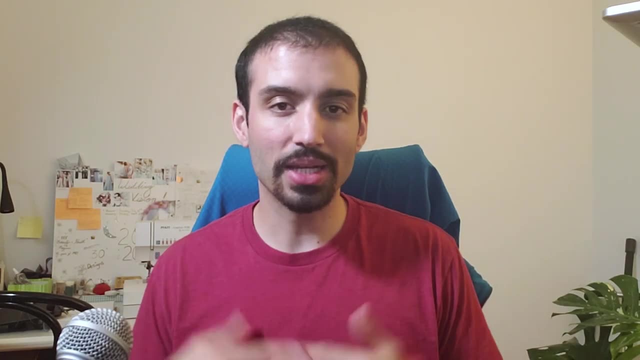 time, the more dependencies that are taken on this service that may exist, the more difficult it gets to change how that service works, at least on the outside. So I guess the truth of the matter is is that it's often going to be very difficult to just throw everything away and start from. 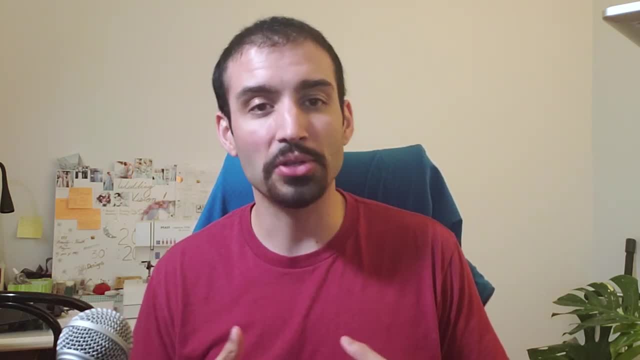 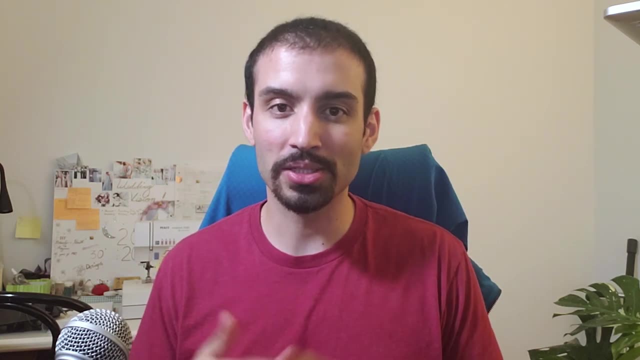 scratch. That almost never happens. Well, I shouldn't say it never happens. It usually happens a couple of times in any organization at some point throughout it. But it's going to be. it's usually a very serious choice. You know it's a cost trade off, analysis of how much effort. 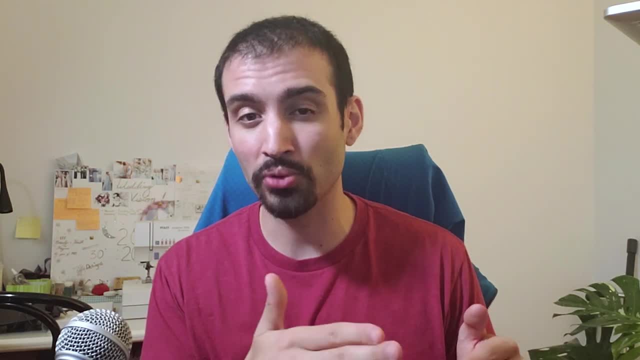 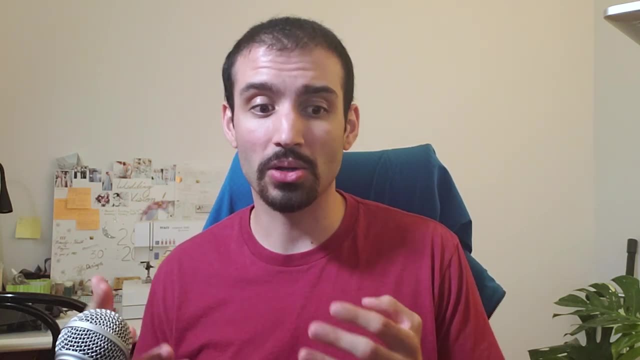 that we put into this thing? how much effort would it cost to maintain it, improve it, versus just starting from scratch? And usually what you'll find is starting from scratch is really the nuclear option. So all we can really fall back on is just improving our existing systems. 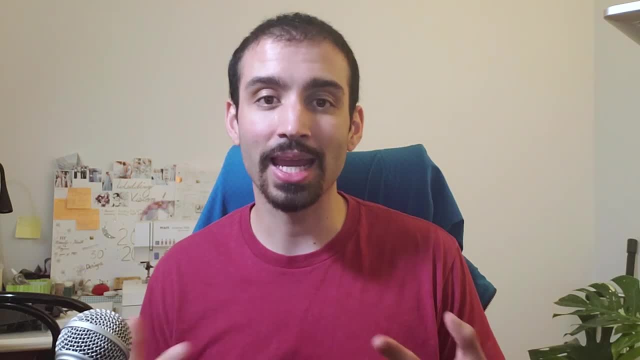 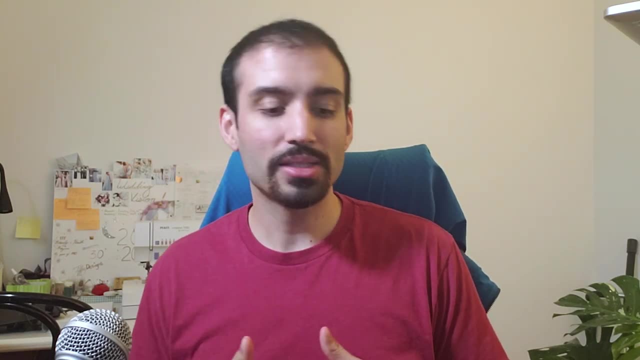 And that's really why refactoring is necessary. We need to maintain and keep the systems that we build healthy, so that they're both extensible and easy to understand for any reader. So that's a little bit about why I think refactoring is necessary Now I just want to kind of share. 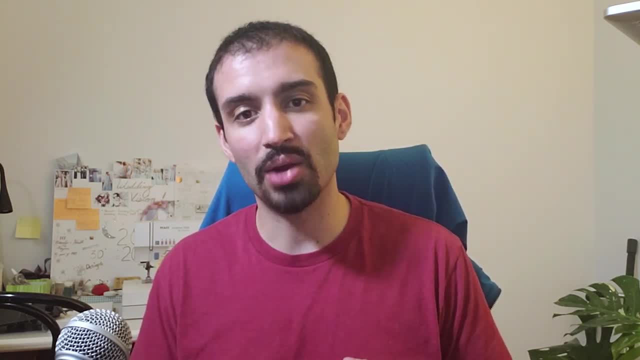 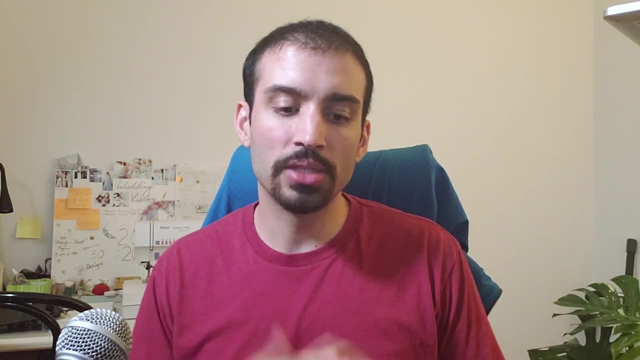 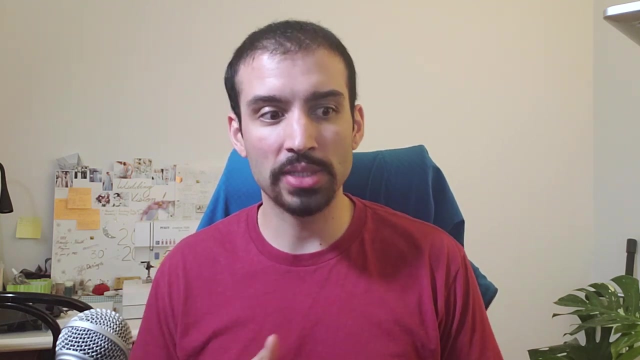 some personal experiences of why I think refactoring is super important. Now I want to kind of latch on to that previous point, which was that often when you build systems they tend to last for a long period of time. My professional experience: I've seen some systems. last for seven, eight, nine years. In fact, a lot of the world's banking infrastructure is still on COBOL-based mainframe systems, So that just gives you an idea of how long systems can last out in the wild. This is especially relevant for like banking and military applications, where 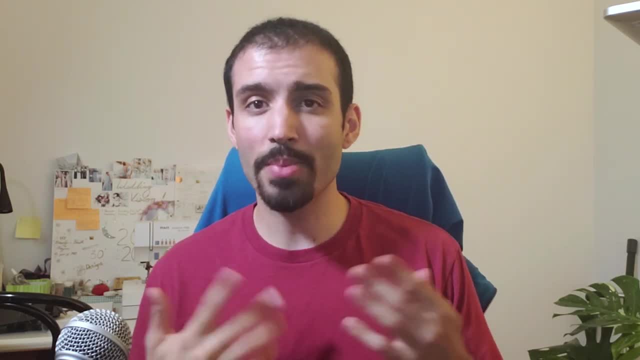 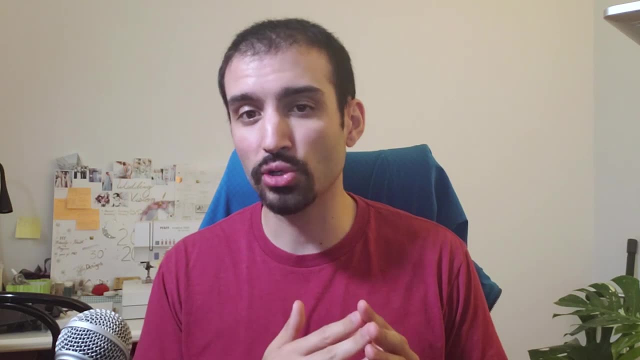 change is usually a very costly exercise. But back into the point: when we originally build our system, we have a certain set of specifications, We have a certain service level agreement in terms of how fast the system is meant to be, how much it's going to scale over time. So the point that 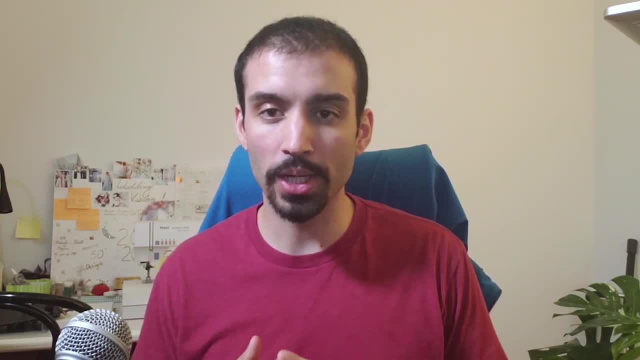 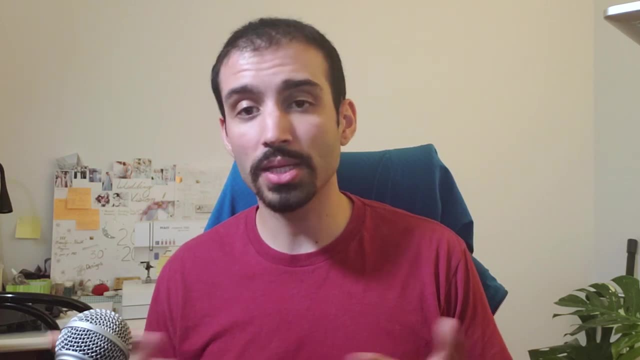 I want to make here is that I think refactoring is a great option. I think refactoring is a great opportunity to revisit past decisions and see if past assumptions are still holding true. So maybe this is in terms of scale, like I was mentioning. Maybe this is in terms of latency. 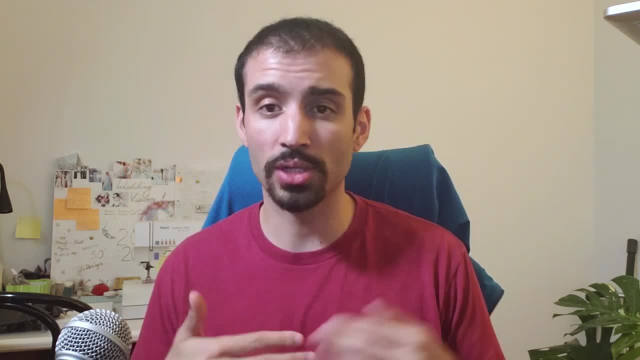 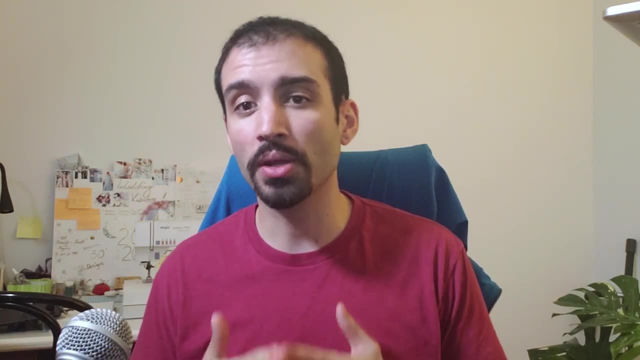 Maybe it's in terms of understanding. It could be the fact that your application has grown and just gotten so complicated that some of the decisions or the patterns that you applied in the past are no longer working for you And it's just taking too long to add new features. 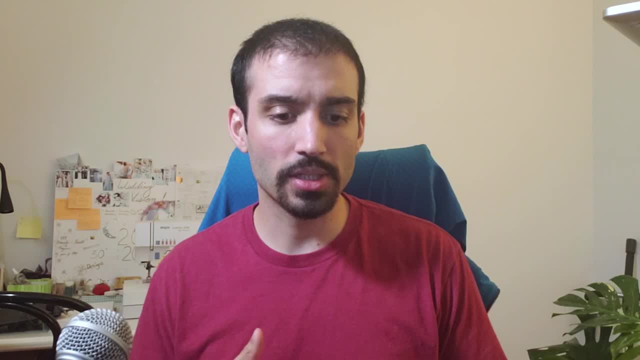 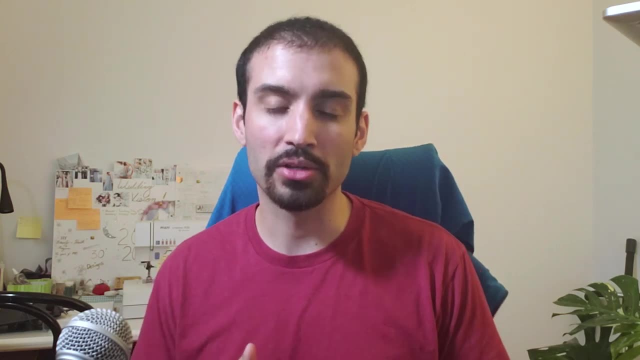 and make changes. So that's my kind of first experience here of why I think refactoring is important. It's to make these long-standing but much necessary architectural changes that allow you to maintain a healthy system. Now the second important reason of why. 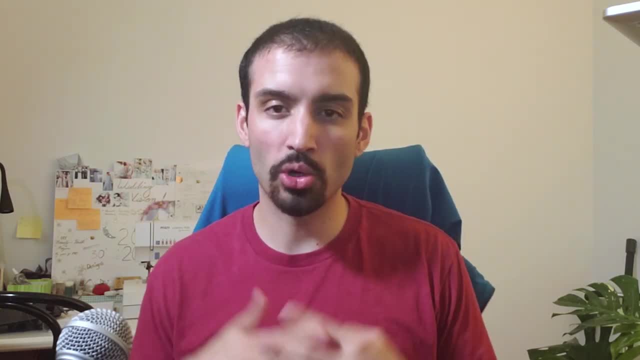 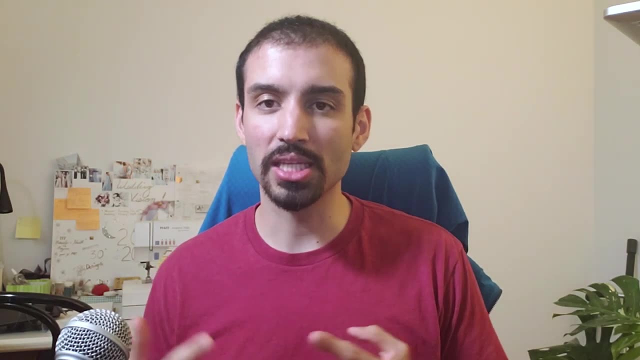 I think refactoring is important is something I like to call domain enrichment. Now, this is kind of a term that I just came up with in this context, But what I mean by it is that when you're on a team and you're maintaining an application, often in the beginning it's very difficult to know what. 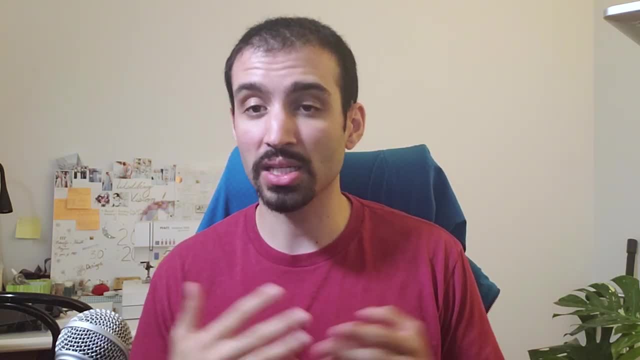 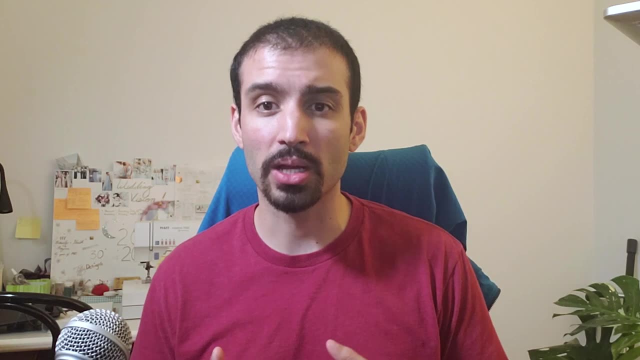 improvements that you need to make in that system. Everything is very foreign to you. You have to maintain it or use it for a long period of time, So it's very difficult for you to tell, as a developer like, what are the pain points of this system. It's only after kind of being in the 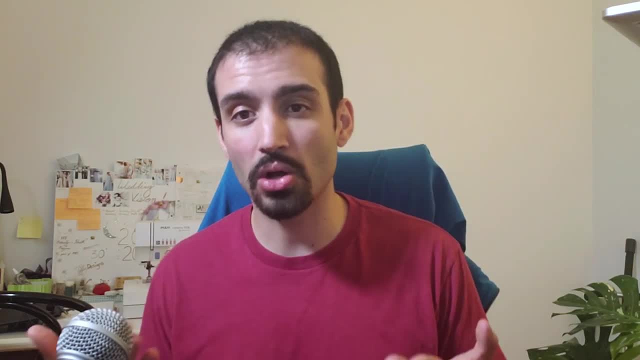 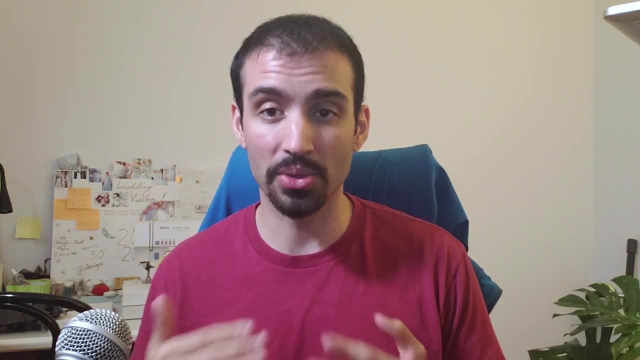 trenches, of owning that service for a period of time. hearing and seeing all those pain points personally, do you really start to get a grasp on what improvements need to be made in the system And when you kind of have these moments of you know this is how the system should work. 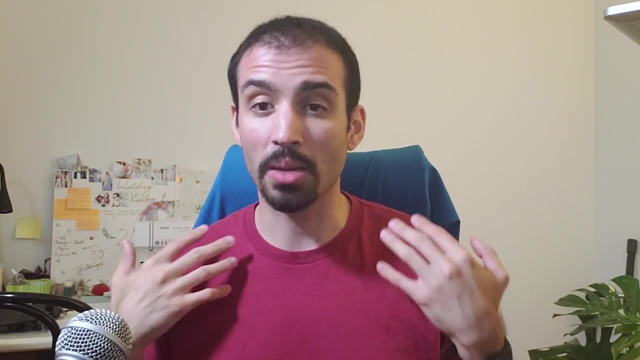 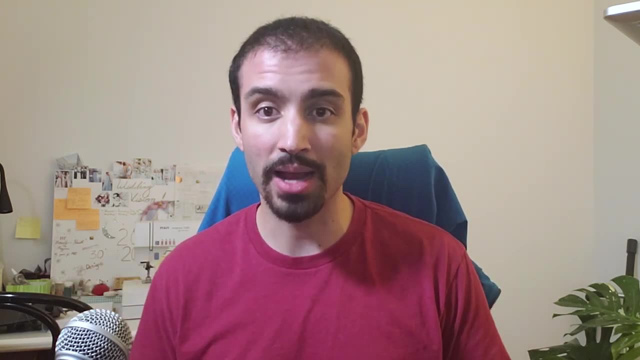 the way we're doing things is completely not working, Like it's completely obvious to me now. This isn't something you can do by just looking at a system from the- you know- bird's eye view perspective, or looking at it from face value. 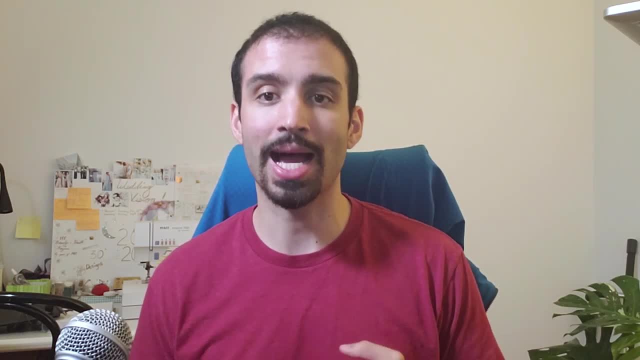 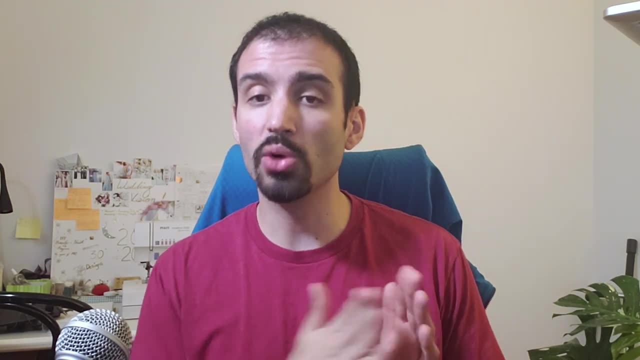 Again, this is something that you learn through an accumulation of time that you spend working with this system. So when you have these revelations that are like: oh, this is how the system should work, it'll make it so much easier for our customers to add new features, Or maybe. 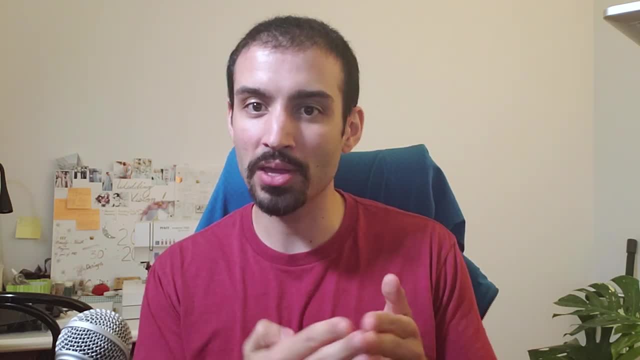 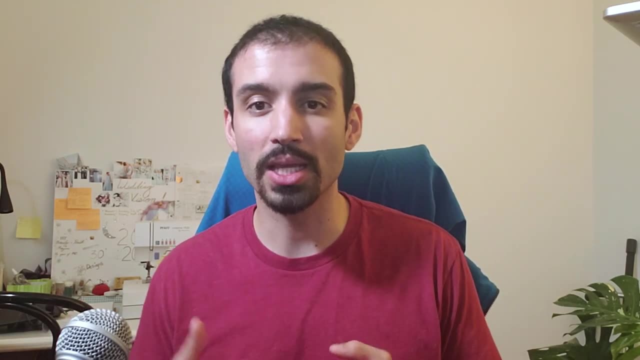 it's a Steve Jobs kind of moment where you're giving your customers something that they don't even know. they want yet Learn things, And I'm calling like. this is what domain enrichment means to me. It's the act of accumulating all this knowledge and learning things about systems over time and using that.